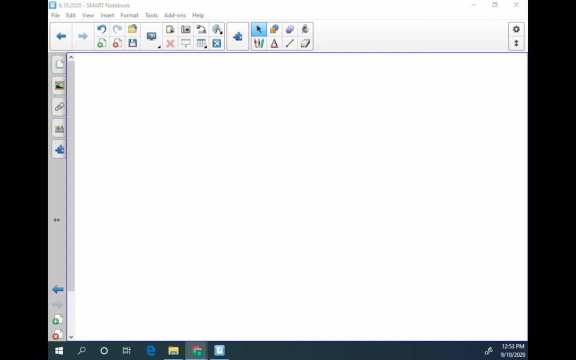 Okay, so we are talking about population growth. Yes, because we talked about what ecology was on the last day that we were here, Tuesday. Y'all described populations with your hybrid assignment from yesterday and today we are talking about population growth, How we measure it, why we care about it and the different types of population growth. that 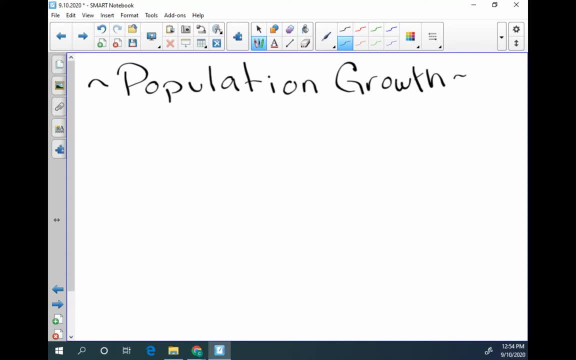 exist in different populations, All right. So Okay, so we are talking about population growth. Yes, because we talked about population growth. Yes, because we are talking about population growth, All right. So there are a couple things that determine population growth. So factors: 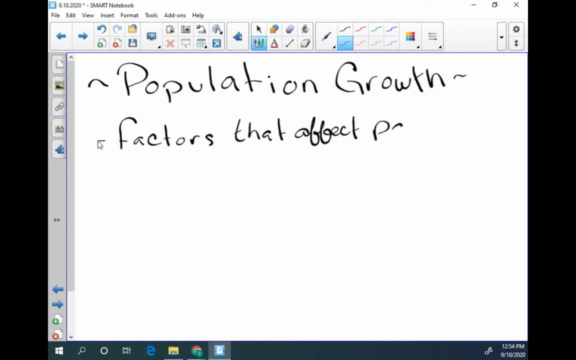 that affect population growth. We're going to write population out a lot, so I'm going to start abbreviating it to POP. You can write out all the population if you want. You can abbreviate it if you want. Do not not care, They're your notes, as long as you know what's going on. The first one we're: 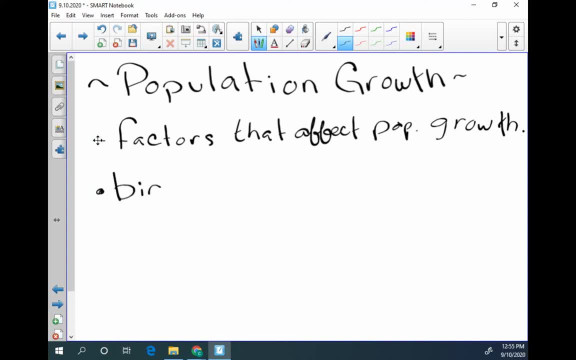 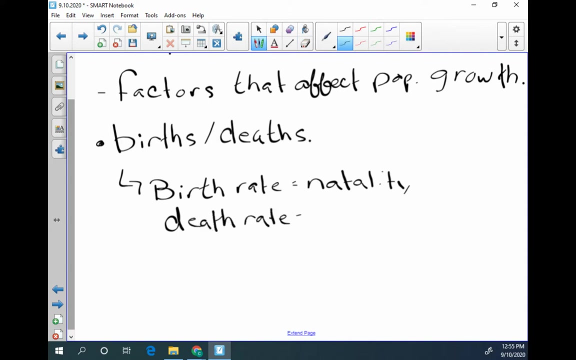 going to talk about is births and deaths. Naturally, our population is going to be affected in size by the rate at which things are born and the rate at which things die. So birth rate is also known as natality. Death rate Is mortality. 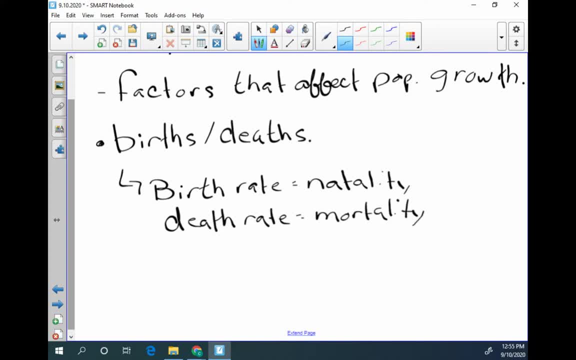 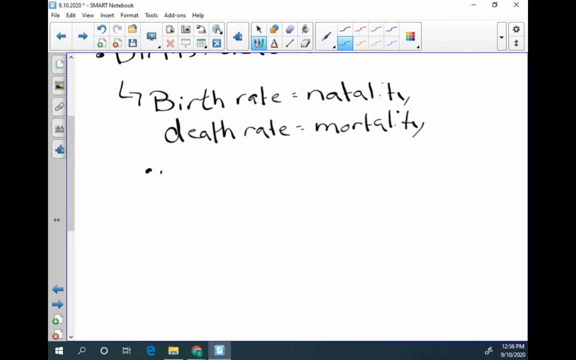 Mortality. So If the birth rate is higher than the death rate, our population will increase. If the birth rate is lower than the death rate, population will decrease. Essentially, if more people are being born than people are dying, then our population is going to. 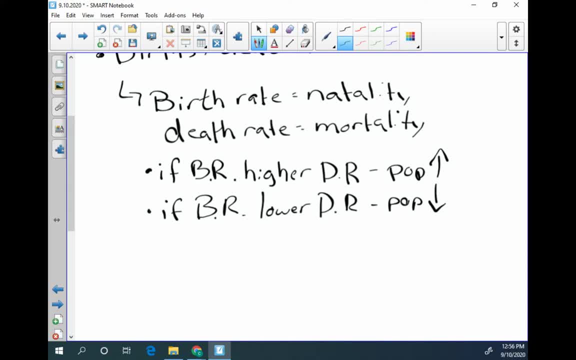 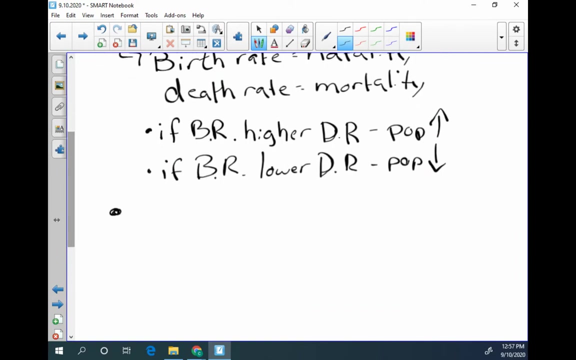 rise in numbers, And if our- uh, if people are dying faster than they're being born, population will drop. The other factor that affects population growth is immigration, and emigration Is faculty learning immigration. Then there's all of these things over view. 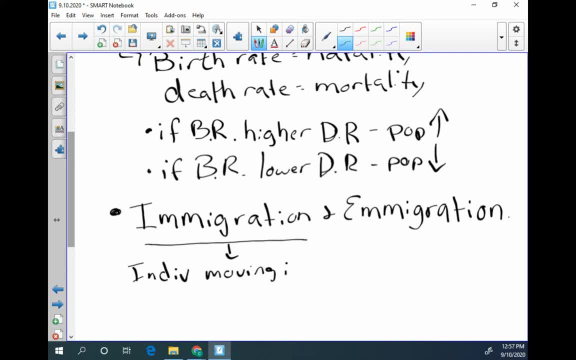 So immigration. Are individuals moving in, So immigration, Imprisonment Also. immigration is a force Including um ха, Immigration Thoughts among and beyond. Are individuals moving out, out, Think M, moving in, Think E for exit. So the rate at which individuals move into. 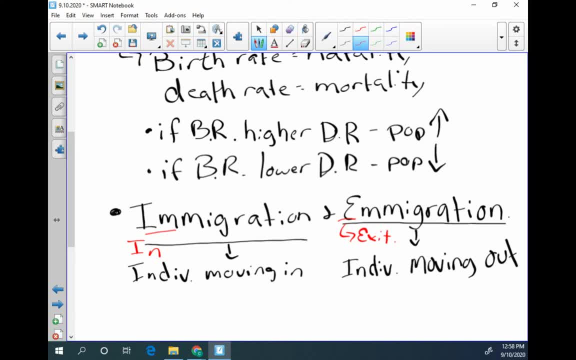 a population and the rate that individuals move out of a population contribute to growth. ie if our birth rates and death rates are stable, like the same amount are being born and die, then our population stays the same. If more individuals are moving in than are. 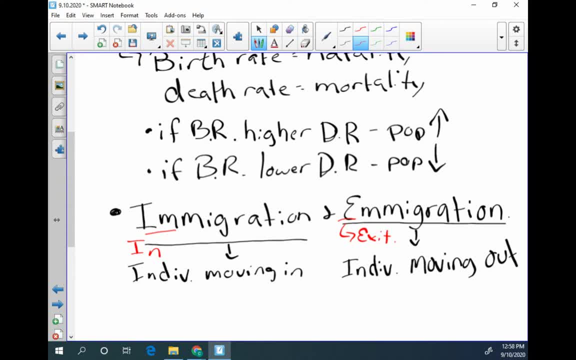 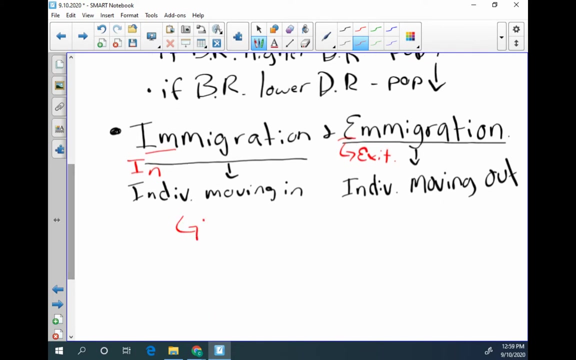 moving out, population will grow, But if more people are leaving than are coming in, population will shrink. Yes, We also have something called migration. If you see, the word migration is in here. Essentially, that is the seasonal movement, seasonal movement of. 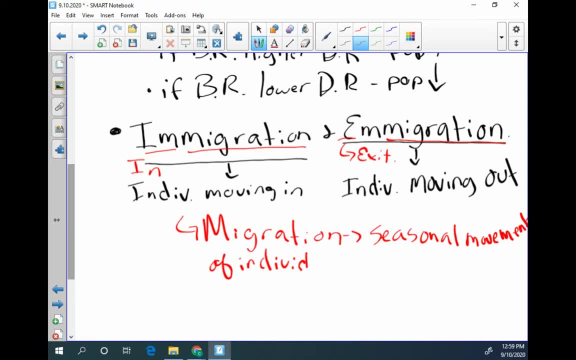 individuals in and out of an area. In the summer our population of Canadian geese is much higher than our population of Canadian geese in the winter. The populations can shuffle and fluctuate over the course of a year, just based on the seasons. When we talk about birth rates and death rates, if we kind of go. 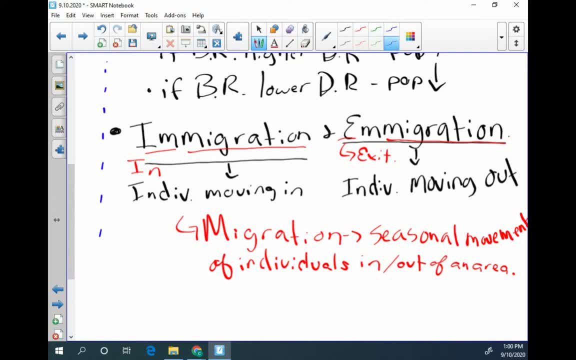 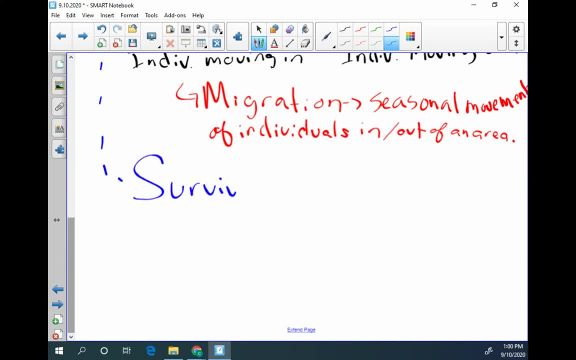 back up and connect this a little bit. we have to talk about something called survivorship curves. Essentially, individuals of different ages have different probabilities of dying and that can be modeled with a survivorship curve. So survivorship curve models the likelihood of death with age. 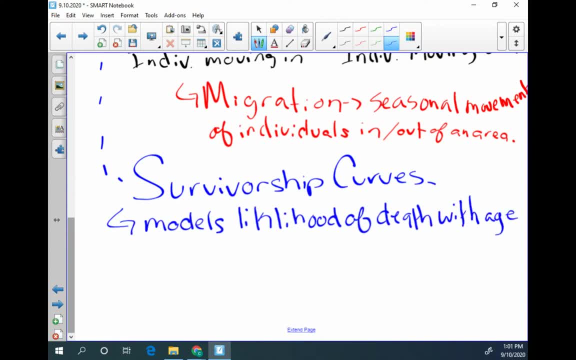 Because, because, because, because individuals at different ages have different probabilities of dying. Individuals at different ages have different probabilities of dying. There are three types of survivorship curves, Three typical models for the rate at which organisms die, based on their age. 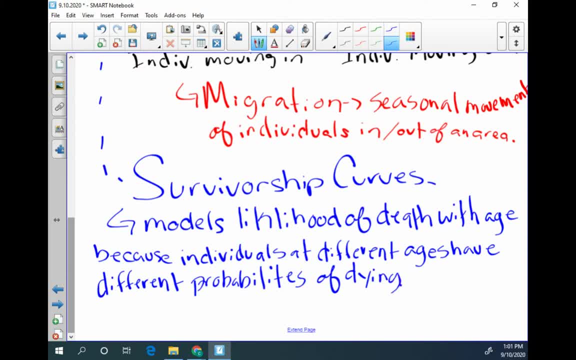 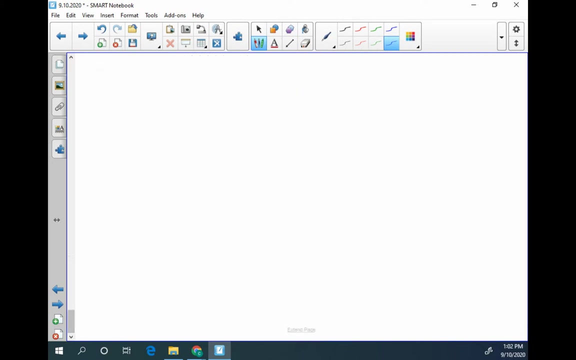 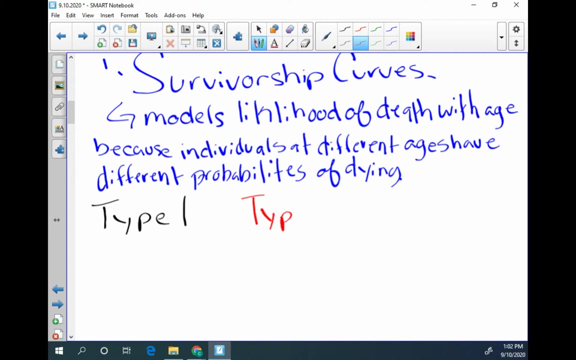 There are three types of survivorship curves, Three typical models for the rate at which organisms die, based on their age. So so, Type 1,, Type 2, and Type 3.. Type 1,, Type 2,, Type 3.. 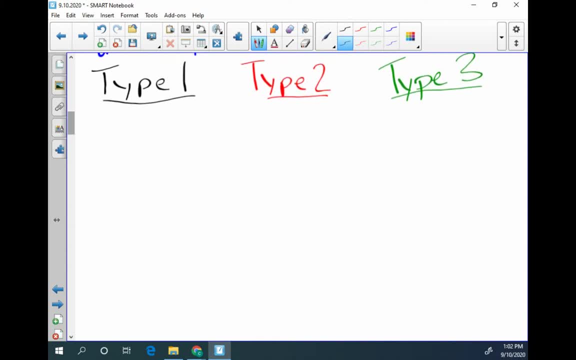 Type 5, Type 6, Type 7, Type 8, Type 8, Type 9, Type 10, Type 12, curves: we are talking about graphs. So actually we'll do it in blue, because you're all going to be the same. 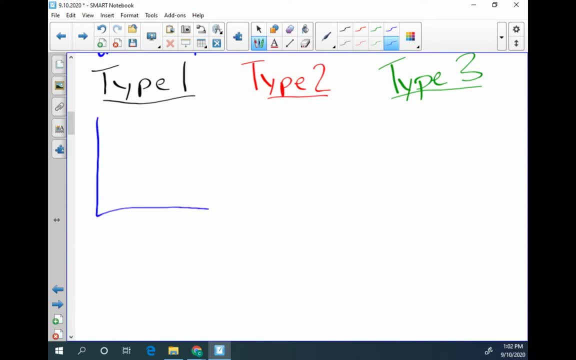 So on the y-axis we have the number of survivors, And on the x-axis we have age. going this way. Now here's a question, Can I? Oh, Okay, Oh, my goodness, I'm a technological giant. This makes me so happy. All right, So we've got our three types of survivorship curves. The first one, our type one survivorship curve. The second one, our type one survivorship curve, is, like humans, We have a type one survivorship curve, meaning that mortality, so death rate, increases with age. 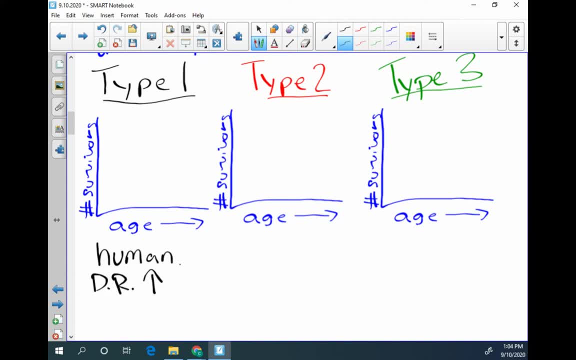 Death rate increases with age. So it looks kind of like that. That's type one. So when you're young, you don't, you have a. there's a lot of young people, a lot of young survivors As you get older. as you get older, as you get older, your likelihood of dying increases, which means we have less old people than we have young people. 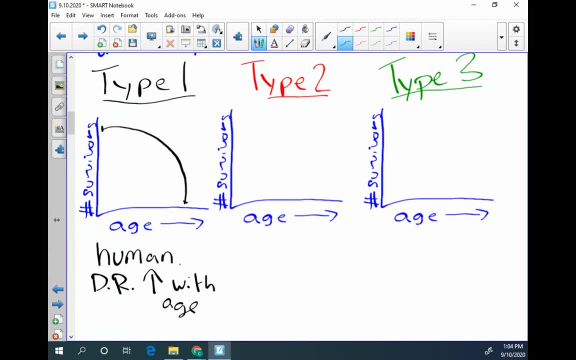 That's typically how it goes anyway. Type two survivorship curves are like birds. A lot of birds have type two survivorship curves, meaning the death rate is equal at all ages. You have the same likelihood to die As a chick as you do as an old bird. 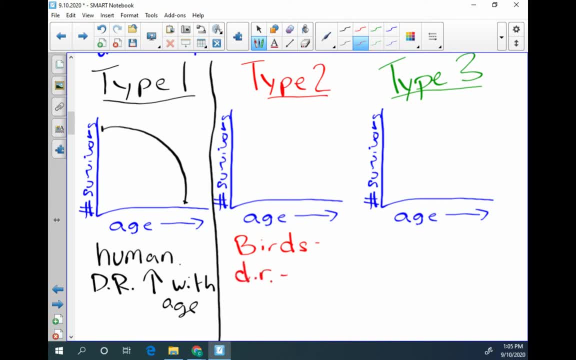 So death rate equal at all ages. So it's just a straight line down, Same rate of death, which means that as organisms get older there's less and less of them, but that pace is the same, Meaning: between this point and this point, the same number of people died. 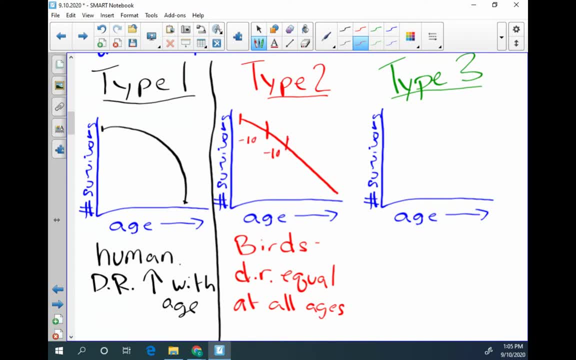 So let's we'll say: there's 10 birds there, 10 birds there, 10 birds there. does that make sense? Whereas with our humans we'll say: we lost one here, we lost three here, we lost 10 here, we lost 30 here, if that makes sense. 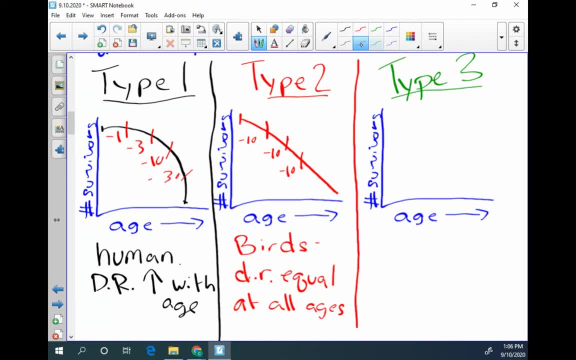 Okay. Type three survivorship curves have a higher rate of death at a young age. High death rate at a young age: This is usually in organisms that have a lot of babies, Like toads. Toads Meaning one mama toad could have like thousands of eggs, right? But of those thousands of eggs, only a couple of them mature to be like actual frogs. So it looks kind of like that, Meaning a bunch of them die at a really, really young age and only a few of them live into old age. 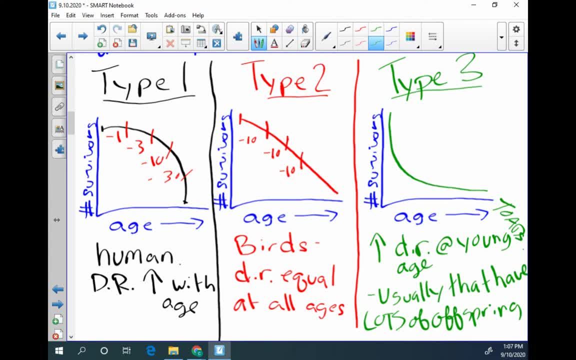 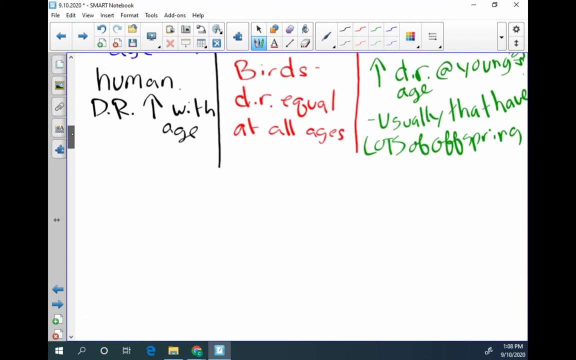 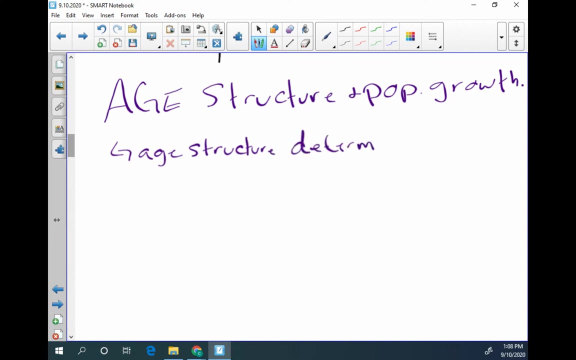 So any questions about survivorship curves, All right. so another- or with this, but another- factor that affects population growth is age structure. So age structure is determined by the relative number of individuals within a certain age group. So 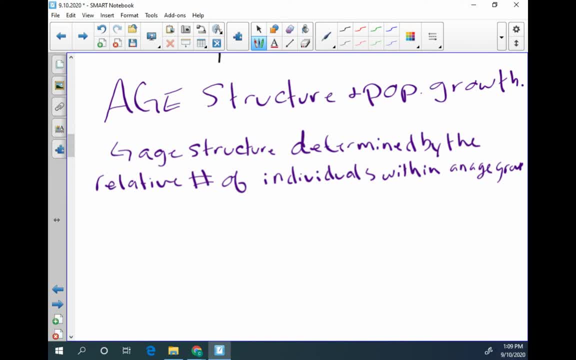 there's a well-known that people diagram these that I'm going to show you really quickly. you will likely see these again, but I just want to show you while I'm talking about it. so this is an age structure diagram, or three different age structure diagrams. the blue is ages- you can't really see it, but like 1 to 14, this is like 20s and 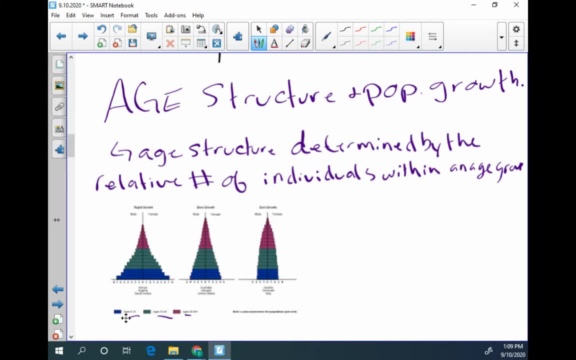 30s, it's like 60s and above. so like there are this many 0 to 16 year olds, this many like 18- 30 year olds and this many certain old people. so this is important, because more young people in a population means that 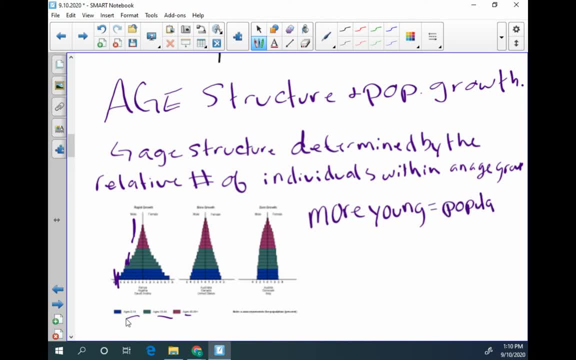 populations are going to increase. more old people population will decrease and if they're even, our population is going to stabilize, which makes sense when you think about it, because if there are like 70 people like our age, but like only 20, 30 people who are like 60s, 70s, we are like age. 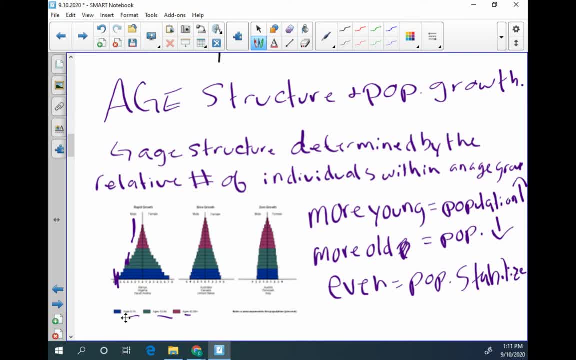 group is the group that will eventually maybe go on to reproduce, but our old people can't anymore. so with more of the population having the potential to reproduce means we are more likely to get more babies. but if we've got like 70 old people and only 20 young people, those 20 young 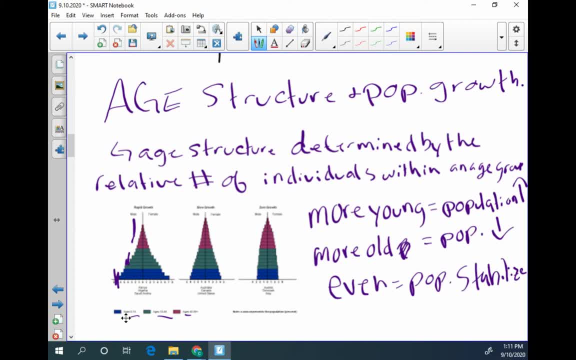 people aren't gonna be able to make enough kids to like grow the population, because those 70 old people are gonna die faster than they can reproduce, and so this population, if this were to like move up, essentially would just go outward like this right, because they would have more babies and they would 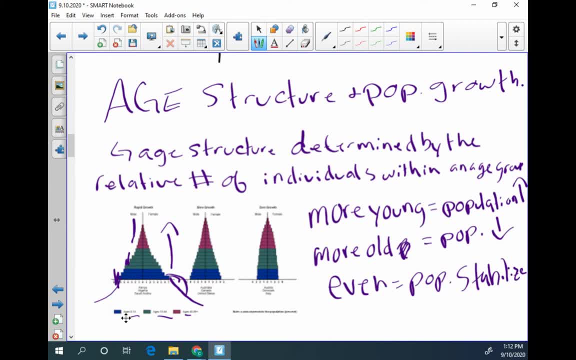 have more babies until they got really big. this one's about stable, but if it were like this, then these guys would all die off and this would eventually funnel out. that make sense. that is a structure. talked about immigration and emigration already. now we are going to. 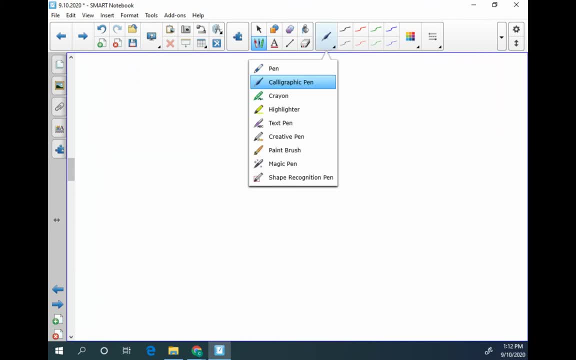 do a little bit of math. so we are going to calculate population growth. calculate population growth so your growth rate equals the individuals added minus the individuals that leave make sense right. So our individuals added is our birth rate. so how many are being born plus the immigration rate? 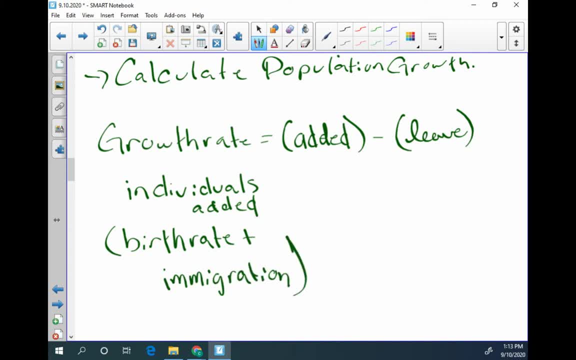 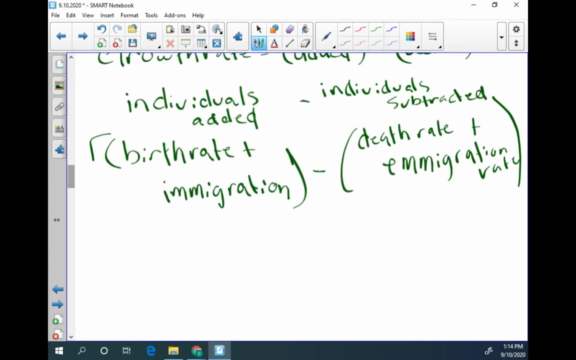 So our two sources of getting organisms or getting individuals are being born and moving in. So our individuals added equals birth rate minus or birth rate plus immigration rate. Our individuals subtracted equals our death rate plus our immigration rate. This will give us our net change in size. So, overall, how many are going to? how fast? 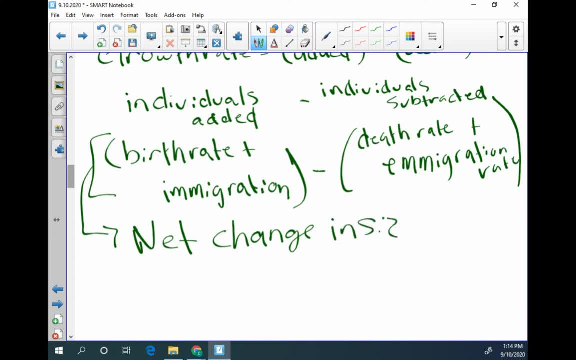 is our population growing. Net change: Net change in size and is usually reported as change per 1,000 individuals. Change per 1,000 individuals. So if overall total, we are gaining seven people a year. we are trying to uh. 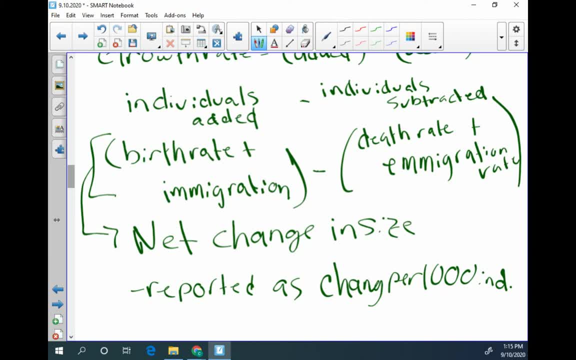 after we get through our birth rate and death rate. in all that calculations we are overall gaining seven people a year. Our growth rate would be seven over 1,000. Or we can do an example. So if we have a population, our birth rate. 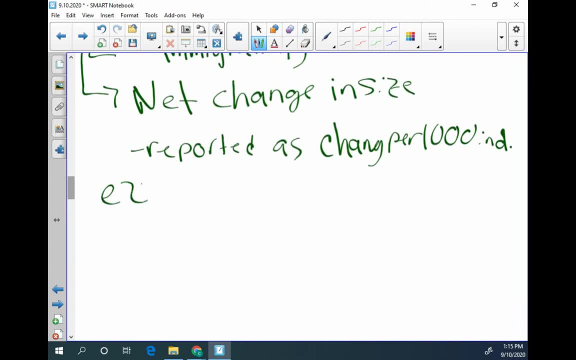 So what we're and we're time and we're counting theれ emails, are we going to necessarily be getting time of life? Not even graôgues Nancy. Thanks, Casey Cool is 18 per 1,000.. 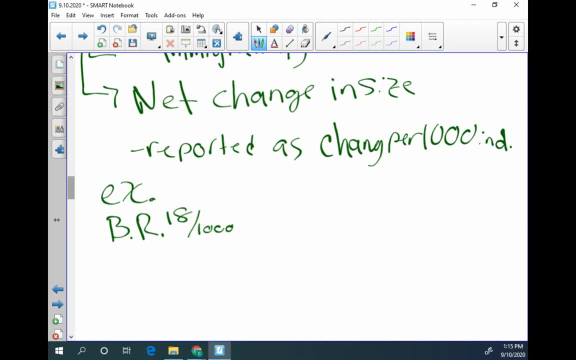 So for every 1,000, let's say we'll use birds- For every 1,000 birds we're getting 18 babies. Out of every 1,000 birds, we're getting 10 deaths. That's our death rate. 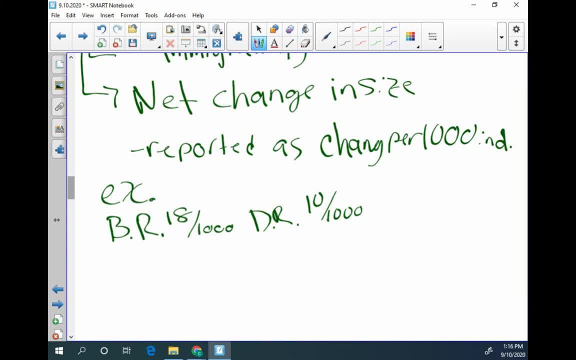 Our immigration rate? we are getting five. So five birds immigrate out of every 1,000.. And our immigration rate is seven. And out of every 1,000 individuals, 10 of them are dying. Five of them are coming in. 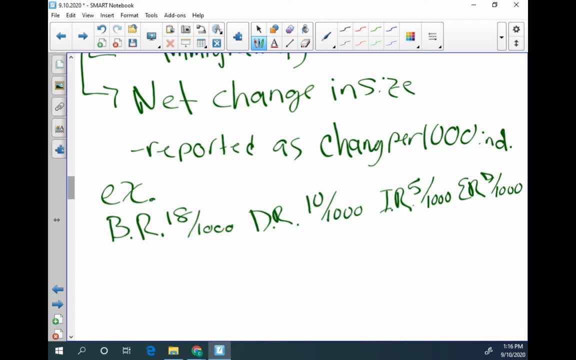 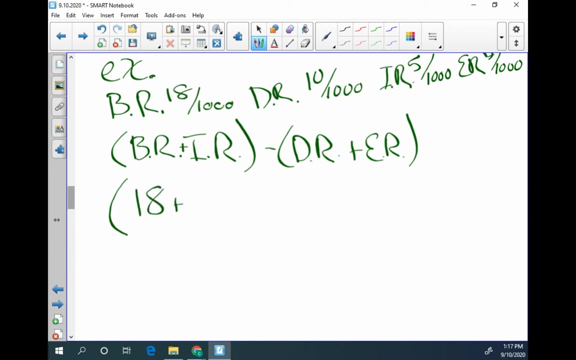 And seven of them are leaving. So remember, we've got our formula, which is birth rate plus immigration rate, minus death rate plus immigration rate, It would be 18.. Plus five minus 10 plus seven, 23 minus 17 equals six per 1,000.. 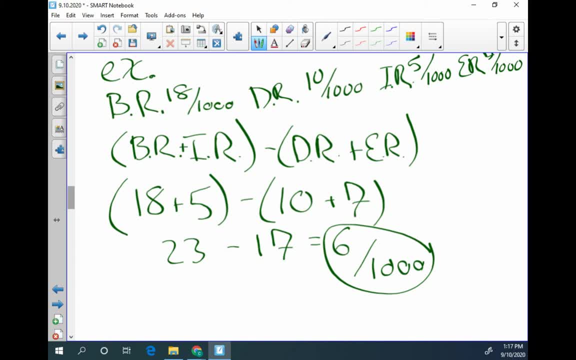 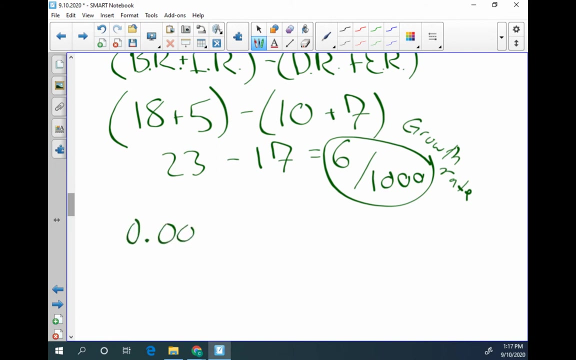 So for every 1,000 individuals on average, we are gaining six. It doesn't matter where from. Our growth rate is six out of 1,000.. Six divided by 1,000 is 0.006.. We're gonna make that a percentage. 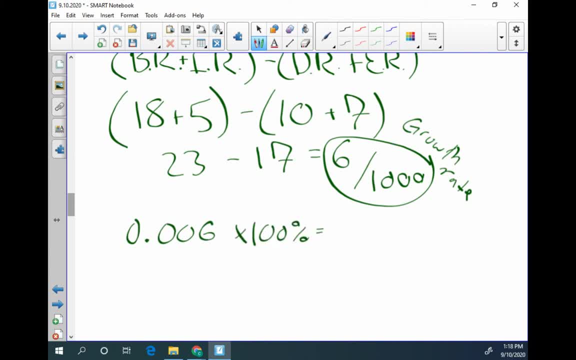 So multiply that by 100% And you get 0.006.. And you get 0.006.. 0.6%, That's our growth rate. Are we following? I know you weren't expecting math today, So now we've got types of population growth. 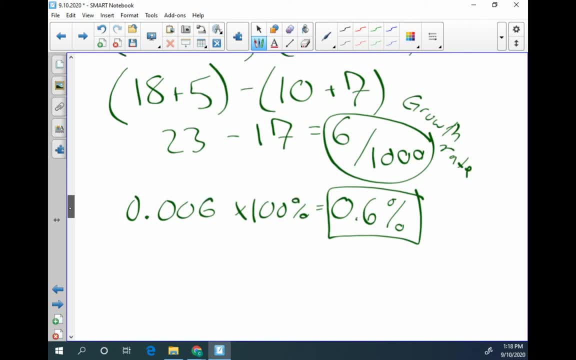 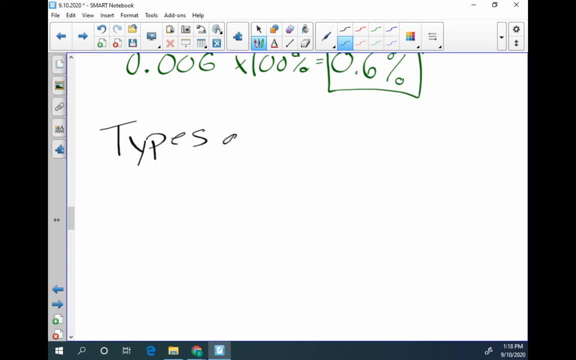 Yes, types of population growth. Where are we headed next? There are two types of population growth, Two types: exponential and logistic. So our exponential growth is where our population grows at a fixed percentage each year. So it'd be like our 6% growth rate right, or 0.6% growth rate. 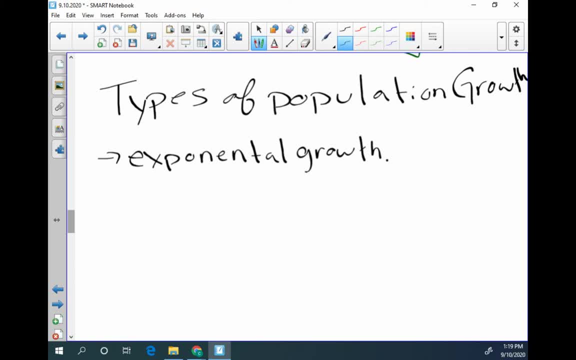 If that was the same every year, if nothing changed and it was always that 0.6%, always that 0.6%, and it never, ever, ever, ever, ever stopped, we would have exponential growth. So population grows at a fixed rate each year. 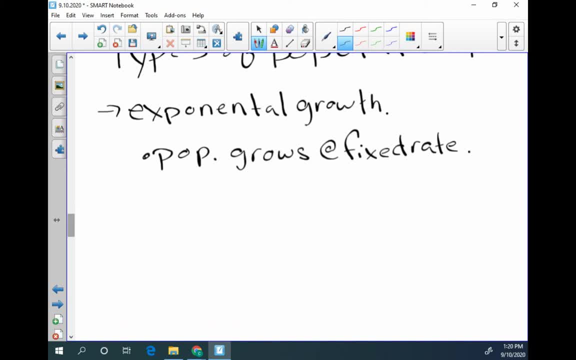 Now, this doesn't happen a lot. Usually, when it does, it is when a population is really small and conditions are ideal. It can't grow forever. essentially, Something's going to stop it. We're going to talk about what's going to stop it. 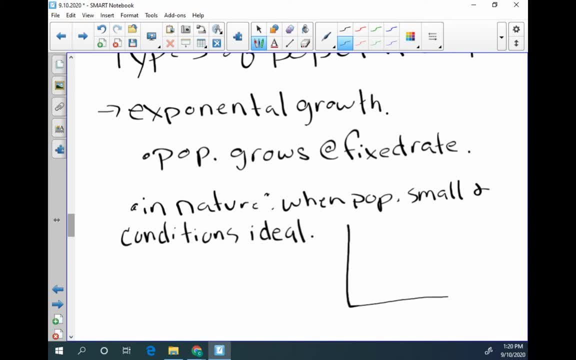 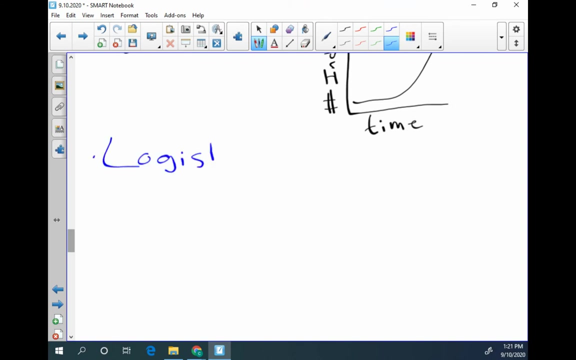 Exponential growth. this is our chart and this is time and this is our population Whoop Straight up. eventually, Much more common, we will get logistic growth. In a logistic growth, the population is restrained by limiting factors. 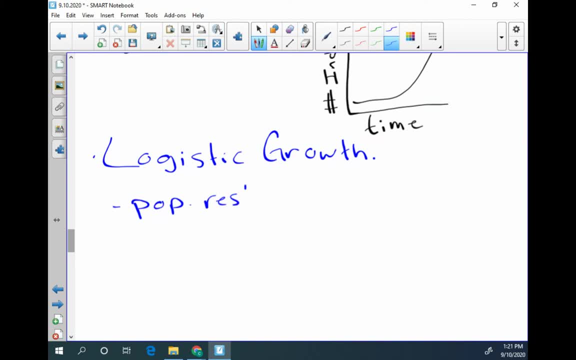 Let's take a look at the chart. We have a graph. Population is restrained by limiting factors. A limiting factor- That's a buzzword. I would highlight that one. Underline it, put a star by it, It'll pop up a lot. 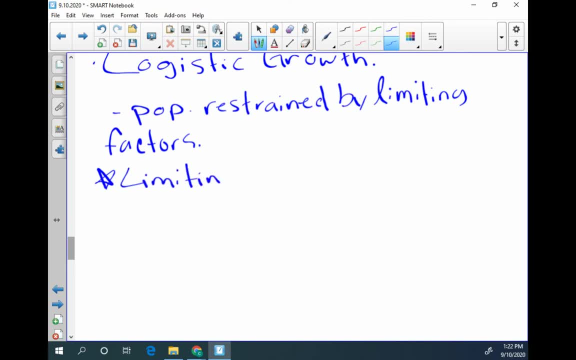 factors are characteristics of environments that limit growth. Characteristics of environments that limit growth. So if we've got our, if we've got a farm and we've got enough space for 60 cows- a lot of space- but we can only feed 40 of them. the rest are going to die. 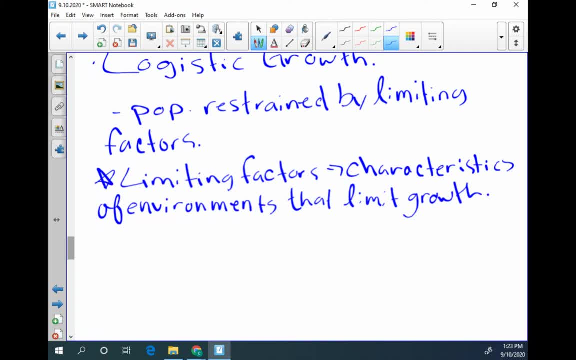 So our food would be our limiting factor. Because our food is dependent on the environment, It's not determining how much, how many cows- we can keep. Limiting factors determine carrying capacity. Carrying capacity is also another one of those buzzwords. 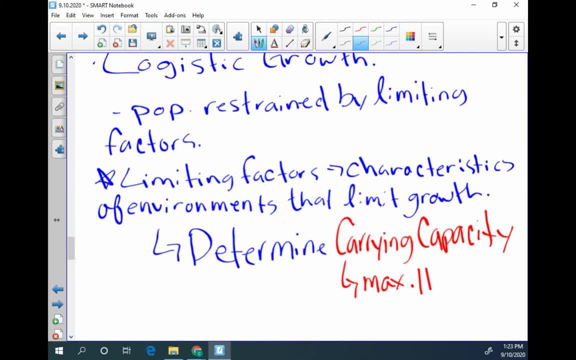 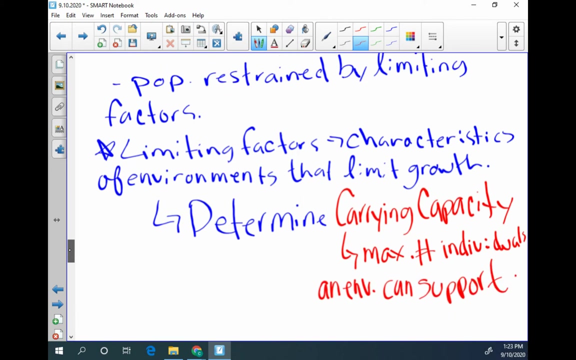 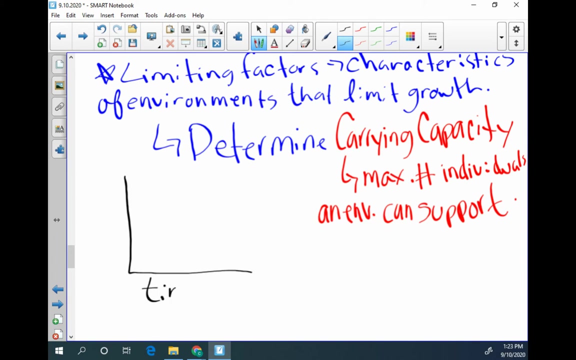 It's the maximum number Of individuals A community or an environment can support, The maximum number of individuals an environment can support. So we've got our chart again With our time And our number of individuals. Our logistic growth Is going to look a lot like exponential at first. 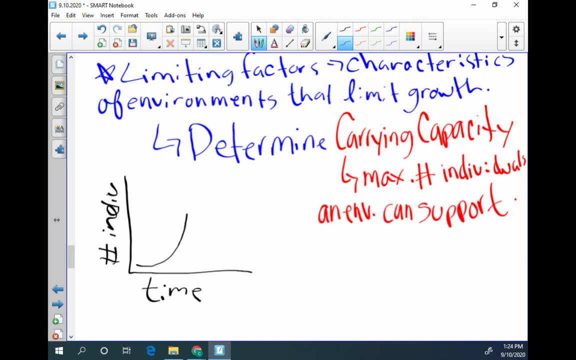 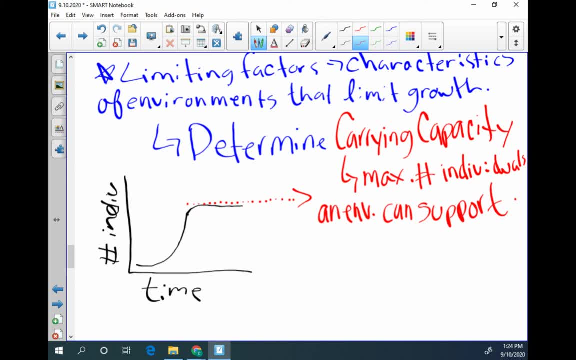 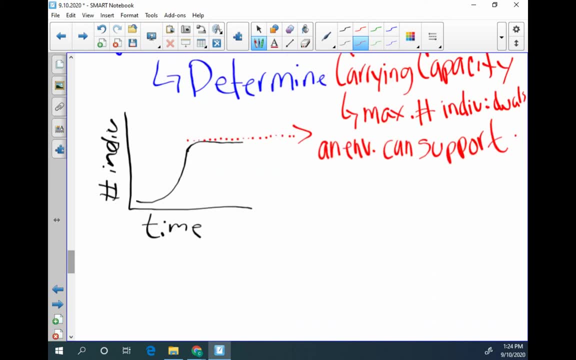 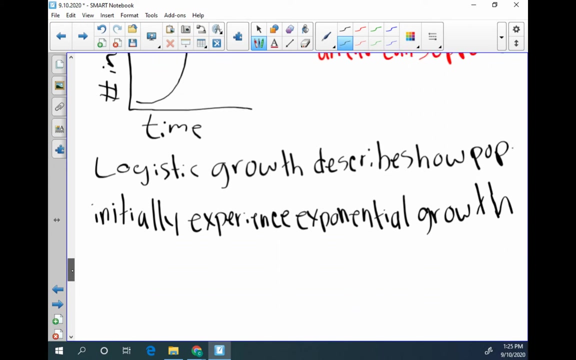 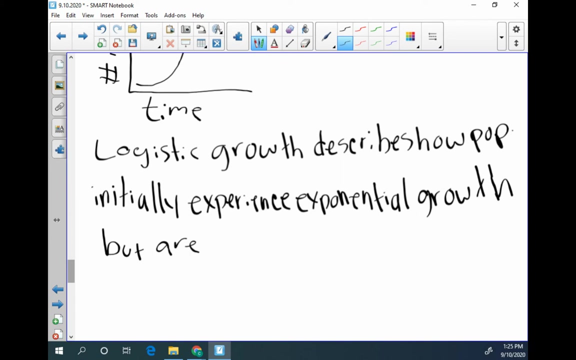 Can't grow no more, Don't have the resources. So if you're looking for a definition, logistic growth. So basically what this is describes how populations initially experience exponential growth. initially experience exponential growth but are eventually slowed and stopped by limiting factors, but are eventually slowed. 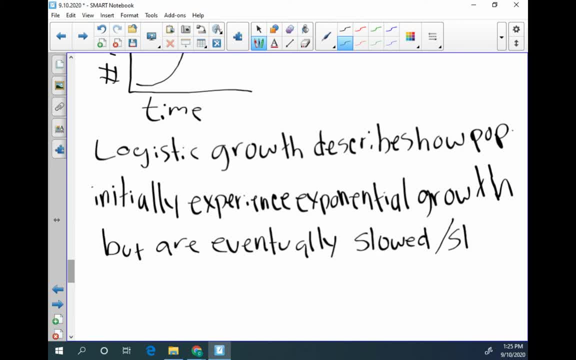 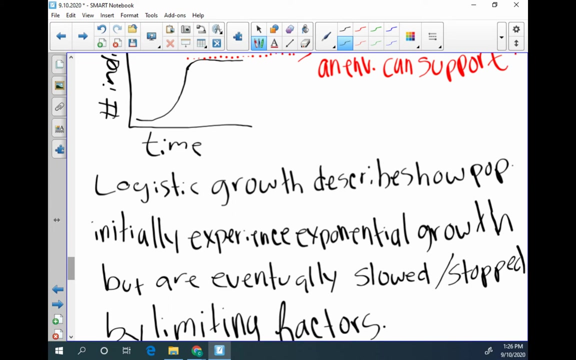 or stopped by limiting factors. by limiting factors, look back up at our graph. we've got our, our period of exponential growth, so our growth rate is fixed, meaning we're just going to keep increasing and keep increasing, and keep increasing and keep increasing until eventually our growth is slowed and stopped. 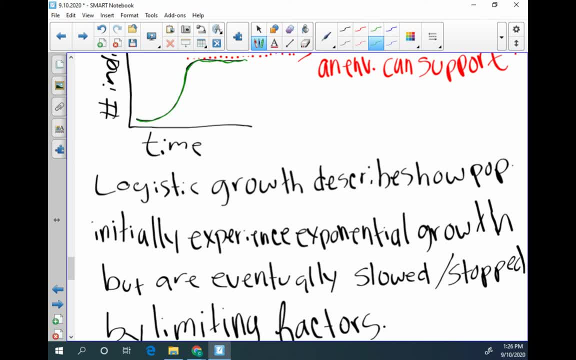 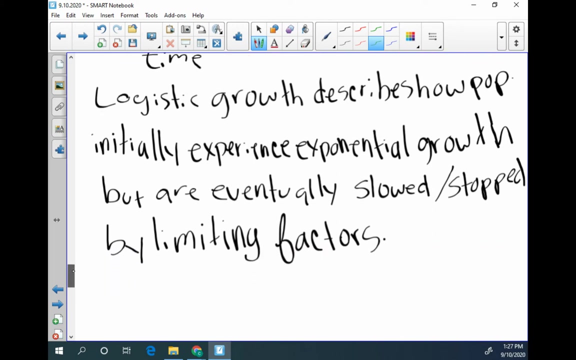 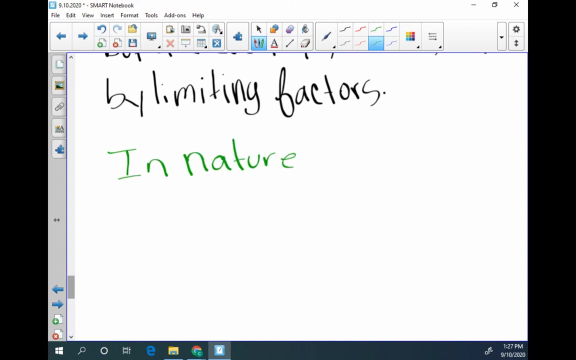 by our limiting factors. tragically, in nature it's not quite that simple. these are excellent models to show us a general idea of what goes on and we can see, but in reality stuff's a little wonky. so in nature populations can fluctuate or cycle through carrying capacity. 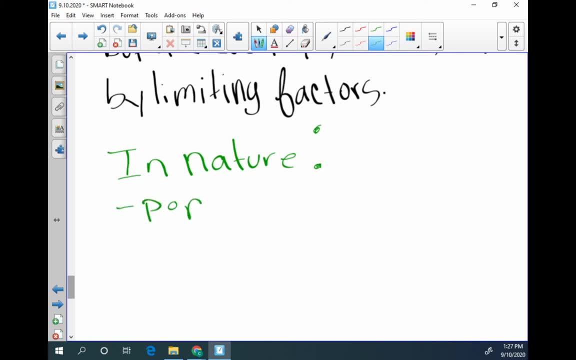 so we can see if this is our logistic growth curve. a lot of the times, a lot of times, we can see that our logistic growth curve is very good. If this was a real population, it can fluctuate, So it'll go up, up, up, up, up, up up. 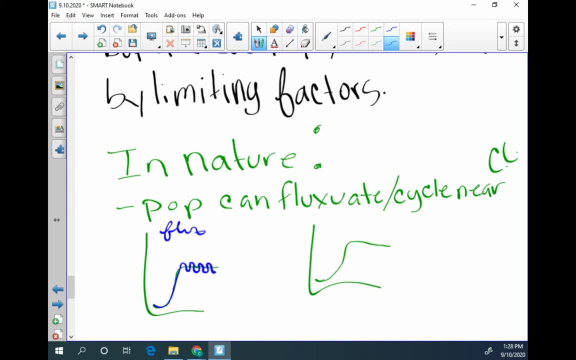 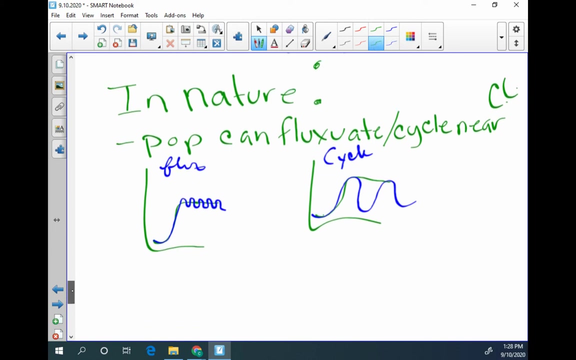 and it'll just kind of flirt with that line, going up and down, up and down, Or it can cycle where it'll go up, reach carrying capacity, come back down, go up, cycle like that, Or they can also rise and crash. 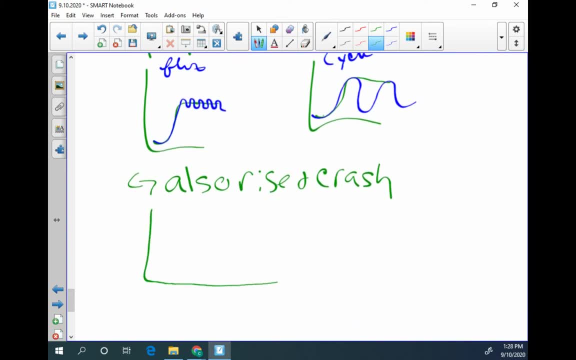 Meaning they can. exponential growth. exponential growth. exponential growth boom. Exponential growth. exponential growth. exponential growth boom. Again, It's not quite cycling, because cycling recovers a lot quicker And a lot of the times the descent is less rapid. 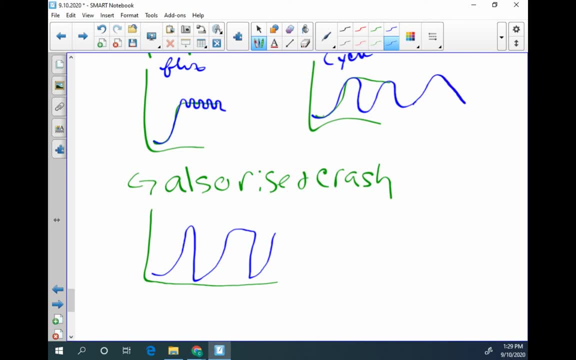 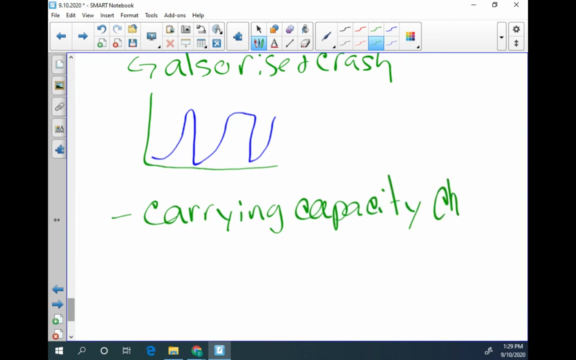 So it'd be like going up slowly coming back down, as opposed to our going up and boom. Another little caveat is that carrying capacity isn't always the same. Carrying capacity changes, So there might be some years where we experience droughts. 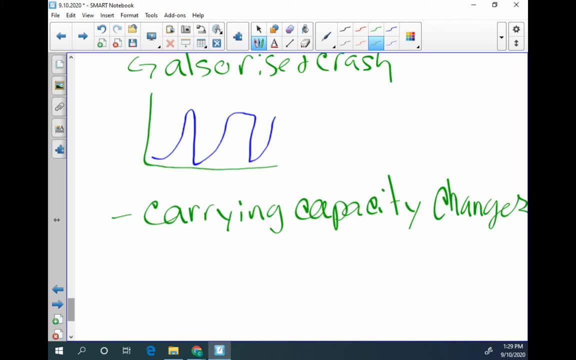 Those droughts would lead to less food, which would lower carrying capacity, Or let's say of a disease- white blood cancer- out a bunch of the wolf population. Well, now those wolves aren't around to eat the rabbits, so the rabbit carrying capacity just shot up. One more thing: We 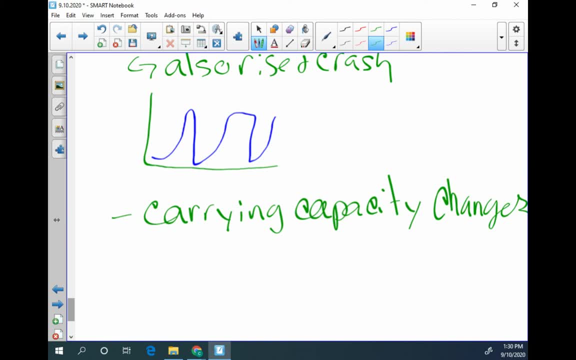 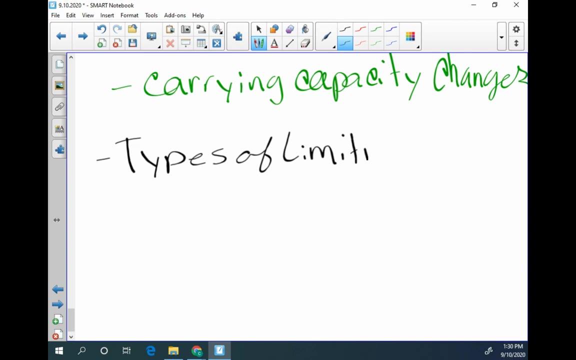 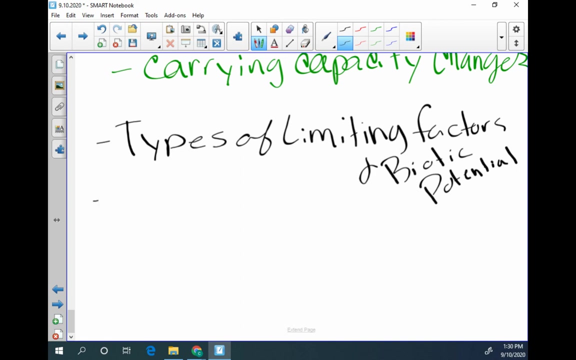 got time. I believe in you. I'm going to talk about types of limiting factors and biotic potential. Types of limiting factors and biotic potential. There are two types, two types of limiting factors. The first is density dependent. The other one is density independent. 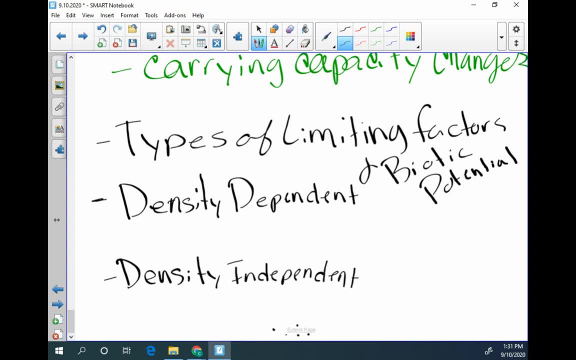 My little button went away. Can I get this page longer? Nope, Alright, so we're stuck in this little bit of thing. So density dependent factors depend on density. Density dependent factors depend on density. That's like competition or disease If there's a lot. 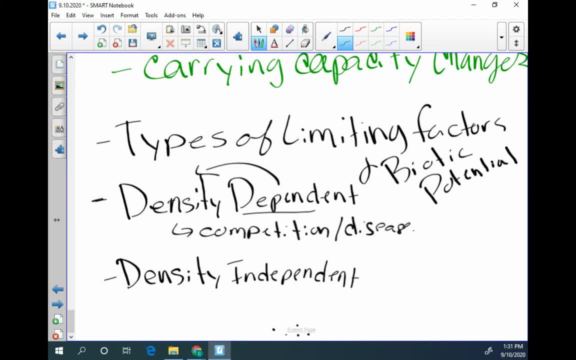 of a population. there's a bunch of organisms packed together. a disease is more likely to transmit through there and it'll take a bunch out. So the bigger the population, the more likely it will have an effect. Competition is the same way. The more organisms that live in an area, the more likely they will have to. 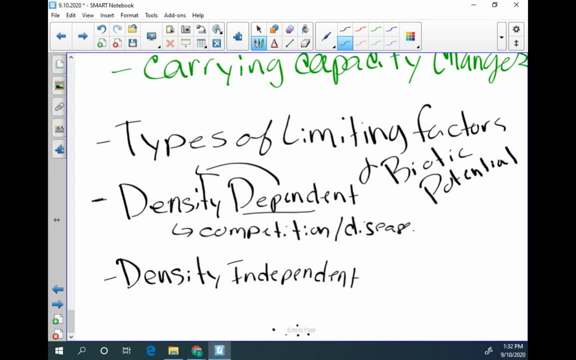 compete for resources. Density- independent factors- are not affected by density, and that'll be like a like our natural disasters. It doesn't matter how many there are. Forest fire is gonna wipe out all of them, no matter what you know. Hmm. 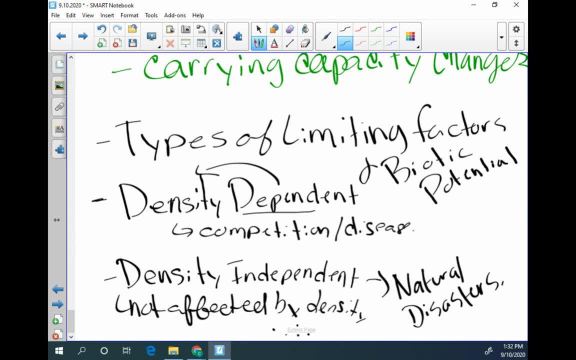 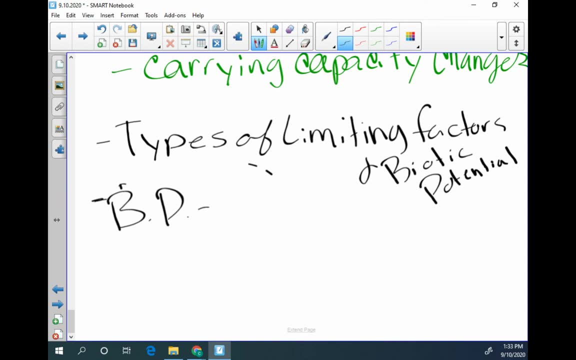 I had to go up and erase a little bit. for biotic potential. You guys have this. Biotic potential is the maximum ability to produce offspring. Biotic potential is the maximum ability to produce offspring. Hmm, Things like how many babies at once? 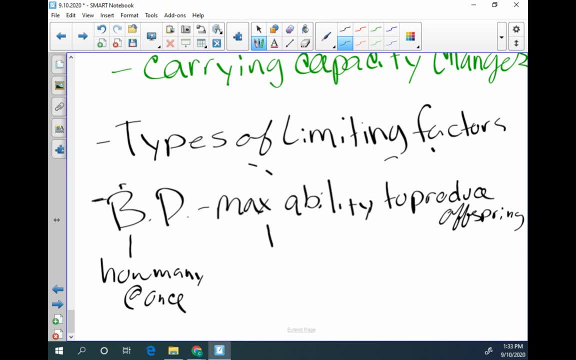 Or how many times can an organism have babies And how long does gestation last? So organisms like those toads that we talked about have a lot of babies all at once. They can do, they can have babies a lot of different times in their lifetime. 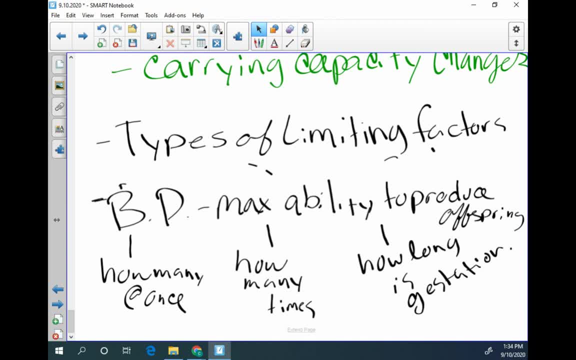 And their gestation or how long it takes for those babies to grow enough to be organisms is relatively short. Or yes, people, for example, have a lower biotic potential because there's usually usually only one, maybe two, occasionally three babies at once.